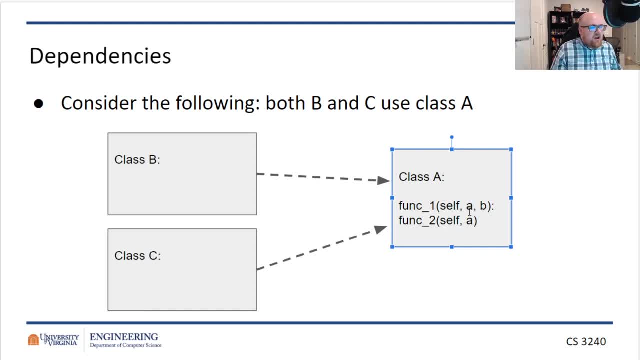 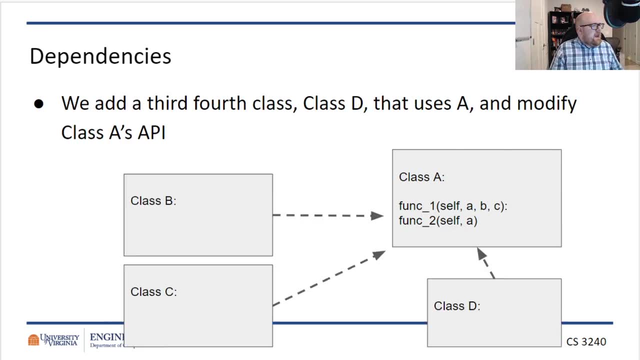 but it's not necessary. If I make changes to the interface in class A, changes to B and C will very likely be necessary, And let's say that we add some fourth class, class D, And class D also uses class A, but because of some extra information, class D needs. 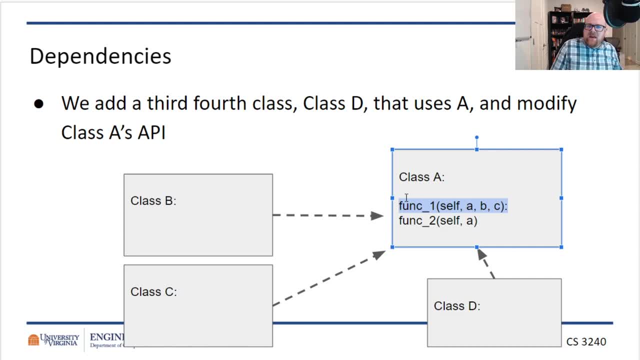 or some extra information it provides. we need to modify the interface of class A, Let's say, add a third argument to this func1 function. Well now, if B and C use this function, B and C have to be updated to include that extra argument. 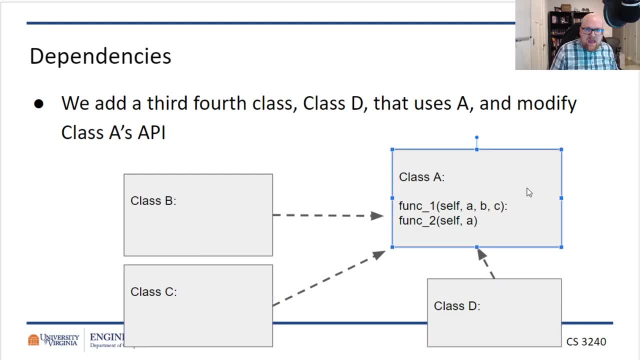 So necessarily by just adding class D to A and making one change to A, I potentially now have to change B and C. Like a still pond, if you drop a stone in it, the water ripples outward. And what we want to do when we build our software is we want to avoid a situation. 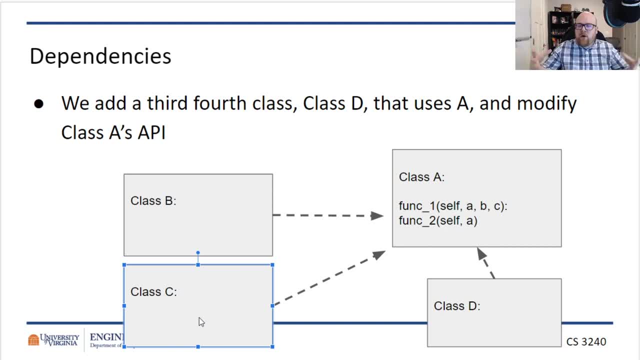 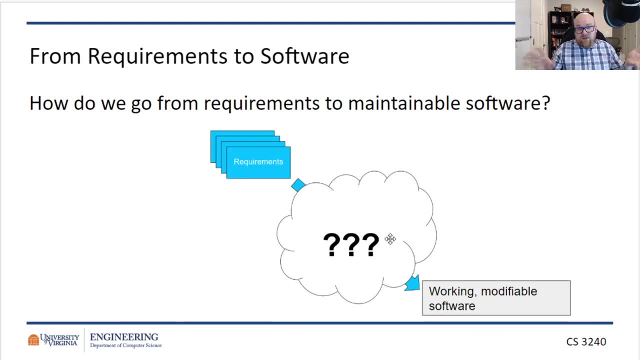 where the pond gets bigger and bigger, and so the ripples spread farther. And so what we want to do is we want to think about design And the first step of design, which is what this is going from requirements to being able to implement a system. 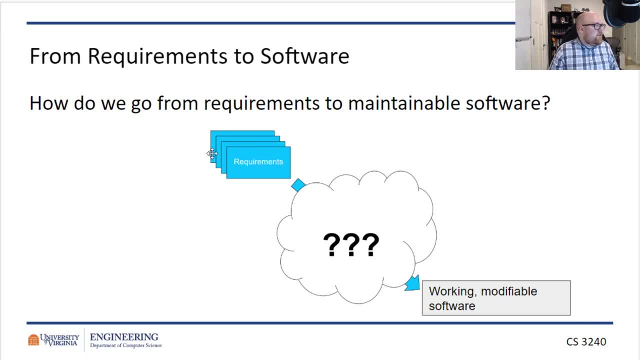 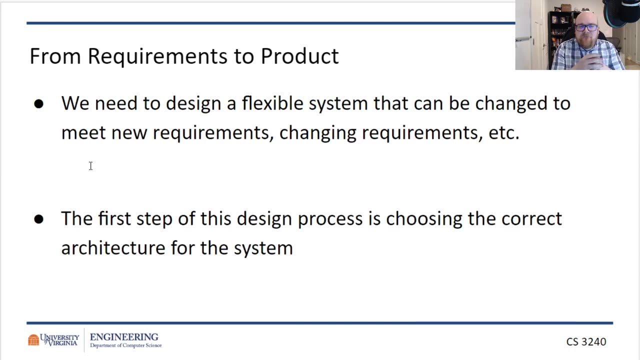 that is what design is going to do. It's going to think about how we build our system in order to ensure the system can be modified later with, hopefully, as little change as possible. So we want to design a flexible system that can be changed to meet new requirements. 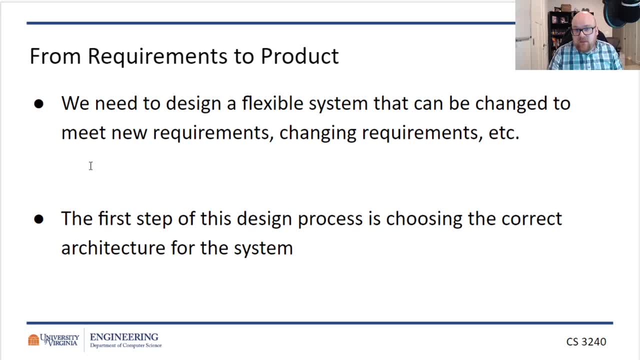 or changing requirements, requirements that aren't initially known, because that's the point of Agile: to be able to respond to that, And the first step of this design process is selecting the correct architecture. You don't just start if we're talking about construction. 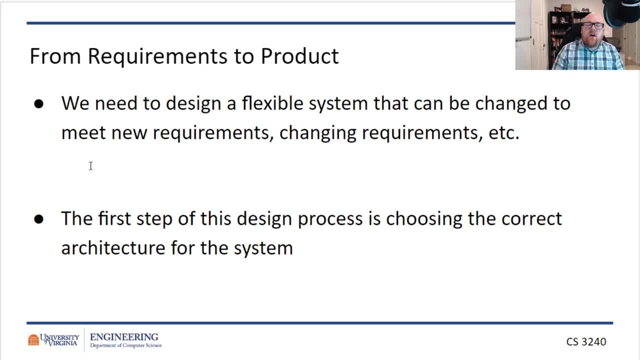 you don't just start building a skyscraper and figure out the architecture as you go. The first thing you have to do is sit down and design the system with the architect, And that's what we're going to talk about. So as software grows, it will be harder to make changes to the existing system. 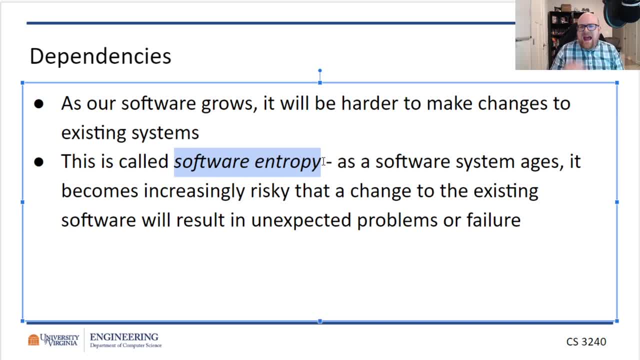 And this is a thing called software entropy, As a software system ages by ages. we don't just mean time by ages, we specifically mean as you make changes to the system, as you add classes, change functions, fix bugs, whatever any changes to the system over time. 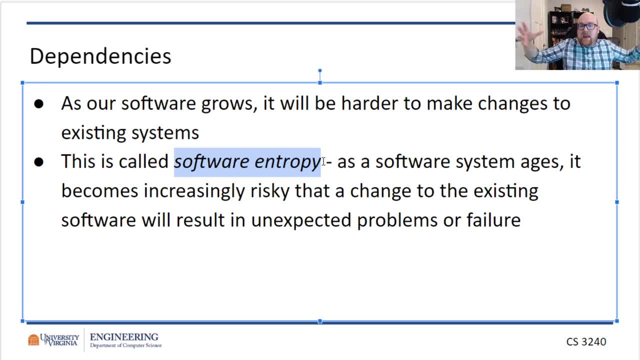 become increasingly risky to propagate, to spread out and cause you to have to change large factors of the system. And having to change other parts of the system to accommodate one change is bad, But it sometimes happens. If we select the correct architecture and the correct design, we can limit that. 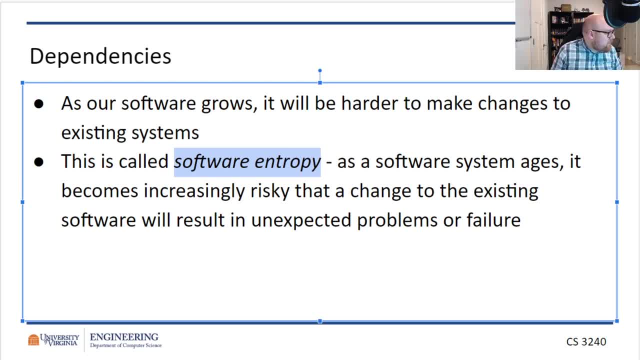 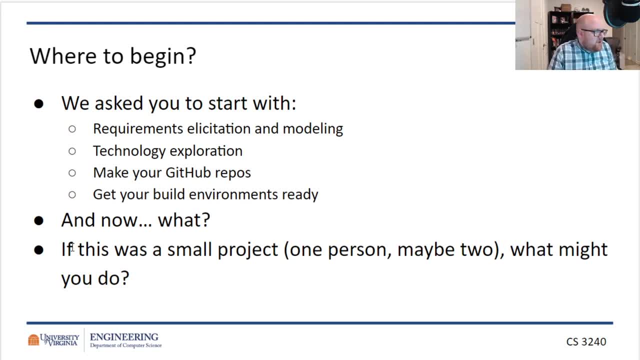 But as our system ages, these events will happen more and more. So where to begin? We've already talked about requirements solicitation. That's our first part. We then want to, and then we talk about modeling those requirements. We then want to do some type of 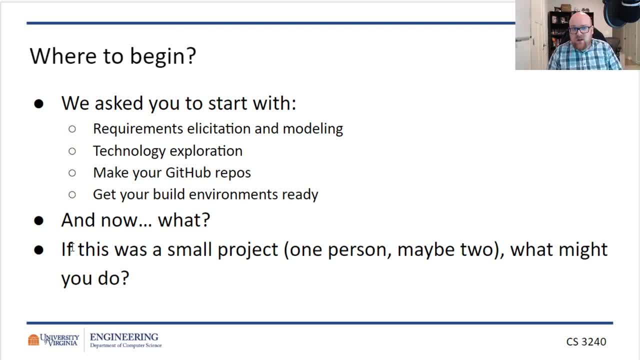 and this is in the case of your project. you've hopefully done this In your project. you've gotten requirements from their survey. Hopefully you've done some type of technology exploration of. here are the things I'm going to need. You know we've talked about using a Google sign-in. 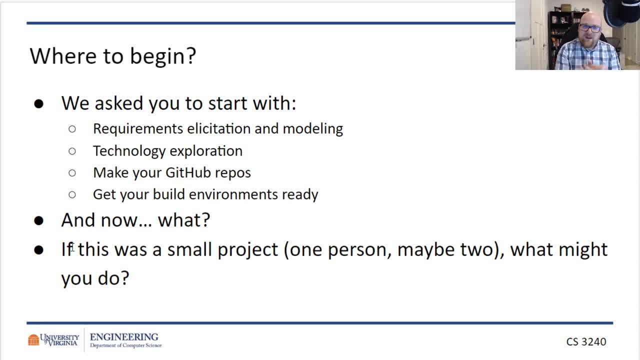 Hopefully you've started exploring that already before you watch this video. You've made your GitHub read of those and you've made your build environments. right Now, what Well, if this were a small project? one or two person, so not, not your group of four, one or two. 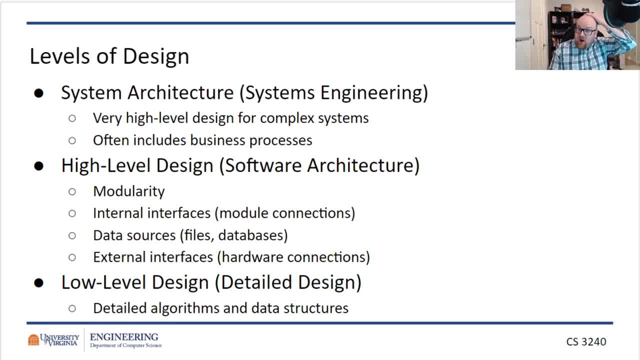 What would you do? Well, you would start by designing the system, and we can talk about design at very different levels. First, we can talk about system architecture. System architecture is very, very high level design of complex systems. It often talks about the business processes here. 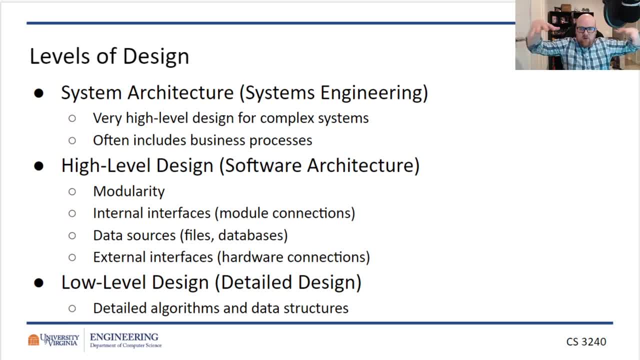 We're talking about, like you know, how the system is going to be used externally, not just within the software. Yeah, who's going to enter, interact with the system? Who are the stakeholders? How are they going to interact? What are they going to do? 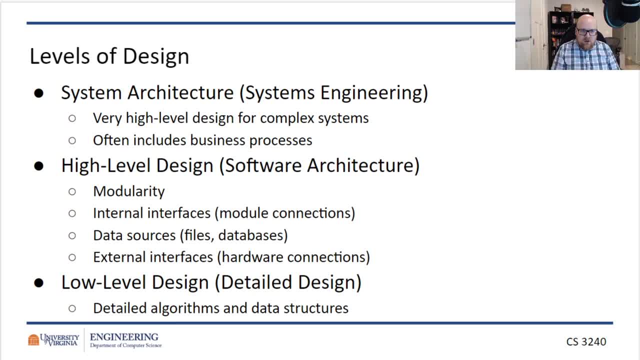 That's. that's talking about the system as a whole. from there We can get into the actual high-level design and we're going to start talking about soon terms like modularity and how that helps Build good software design. talk about what data sources to use, how those data sources are going to be built and interacted with, what internal interfaces are going to exist. 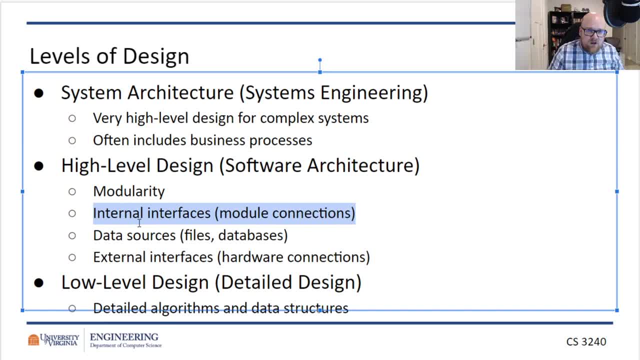 That is how different components interact with each other, as well as external interfaces. How is the system going to be interacted with by the user? Maybe if there's some hardware component, like if you're building an autonomous car- the hardware features need to be incorporated into this design. 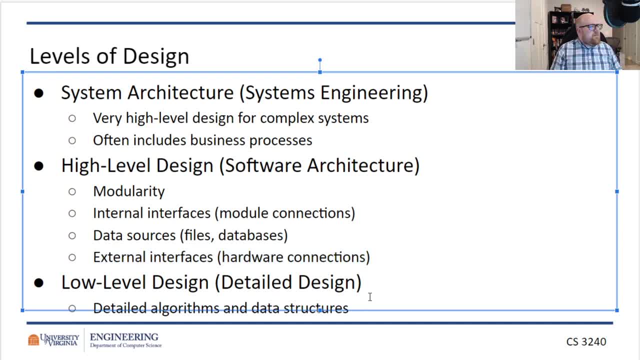 The cameras, Etc. And that's separate from low-level design, because the low-level we're specifically talking about like: what algorithm should we use? What data structures should be used? at high level, We're more talking about, if you think about it in terms of classes, how these classes interact. 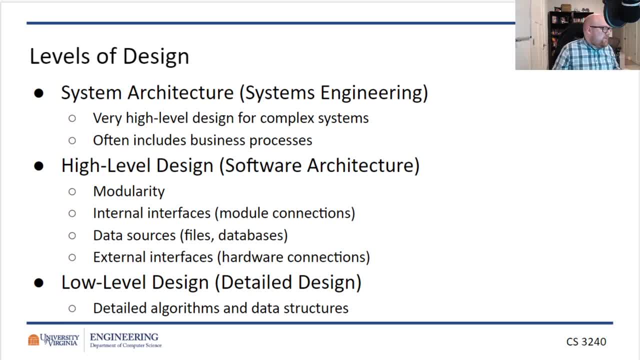 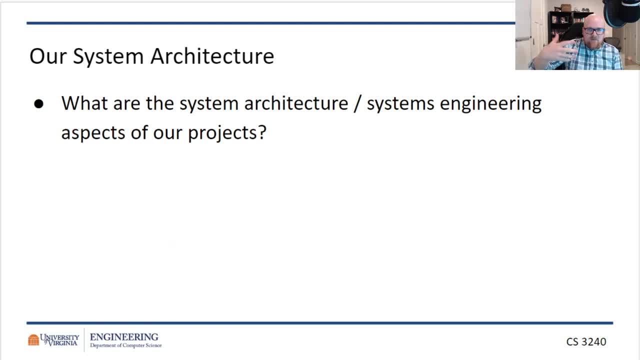 And how groups of classes interact, how groups of classes that form a component interact, Etc. So now, what are the system architecture or system engineering Aspects of your project? pause for a moment and really think about this. Hopefully you started actually implementing something. 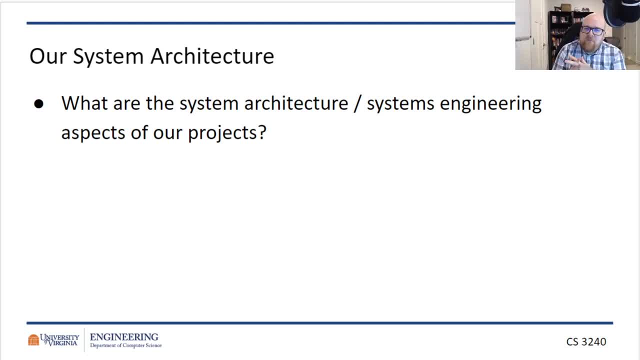 What is the architecture that you have planned, or do you have one planned? What are the system engineering aspects of your project? This is so we so- system architecture, system engineering. We've kind of decided a bit for you, right? You know you're building a Django app. 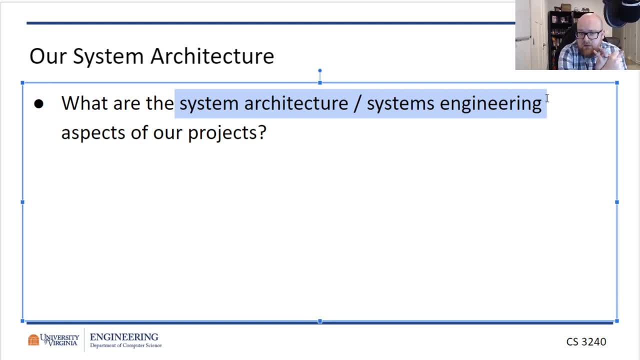 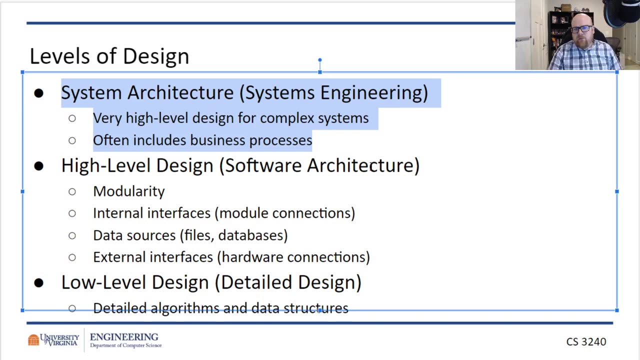 This is going to be used within a web browser, right? Who are the stakeholders? pause the video first here. pause. Pause the video for a second and really think about what are the system architecture points of your system, What are, what are, what is the? who are the stakeholders? 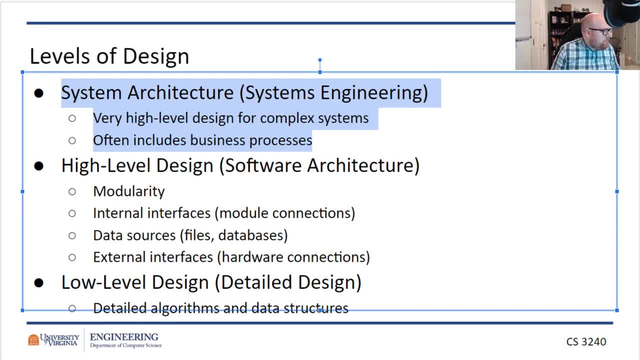 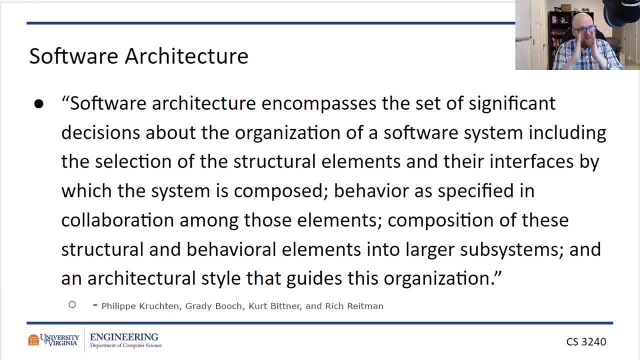 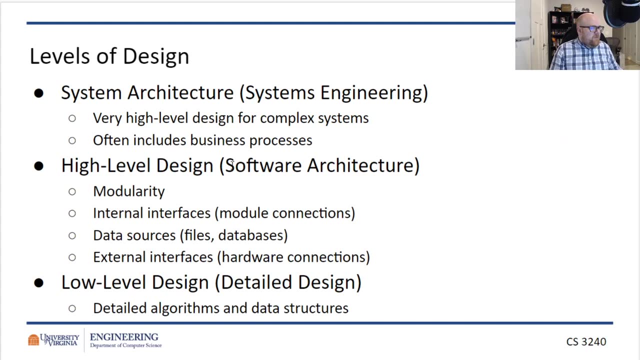 How are they going to interact with the system? Think about that, Okay. But now let's talk about About the software architecture- and hopefully you've paused, If you haven't paused now and think about that, actually really think about it. But now let's get to that middle level, the software architecture, that, that middle level. 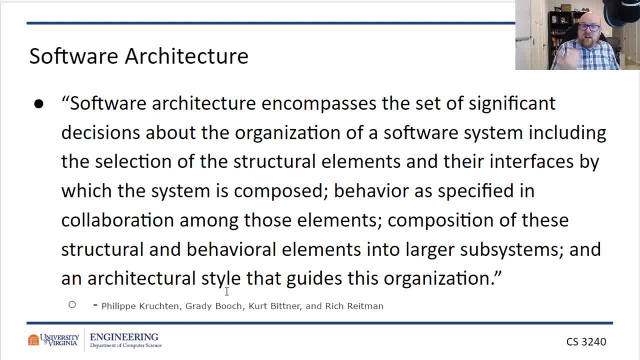 And I'm going to read this quote: software architecture encompasses the set of significant decisions about the organization of the software system, including the selection of the structural elements and their interfaces of which systems compose them. and by interfaces We don't mean user interface Like a, like a website or an app or a command line. 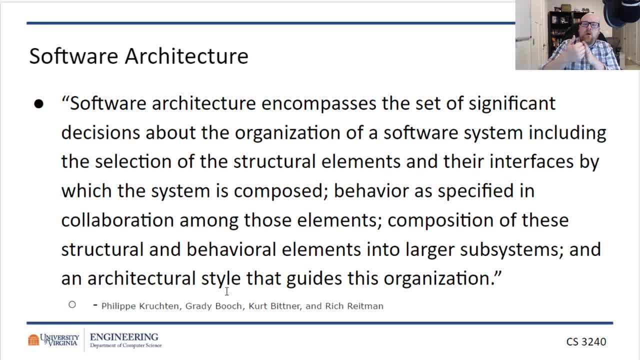 We're talking about the interfaces, in terms of how this component is used by other software within the system. If you remember, back in 2110, we talked about Java interfaces. This is a bit more broad than that. The. the term I would often use here is API. 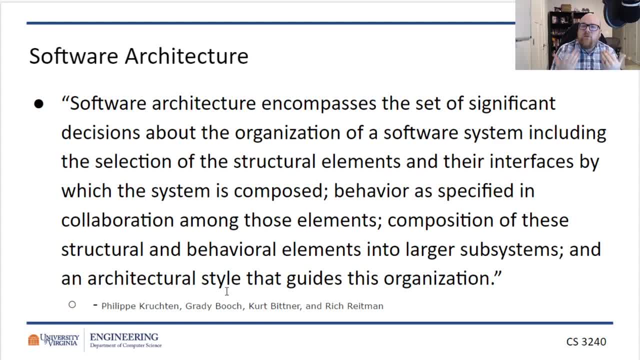 That is, what functions does a class have available? What are those functions do? How are they used? That's what we mean by interfaces In this case. So it's the selection of structural elements and their interfaces, by which system is composed. It is behavior as specified in collaboration among these elements. 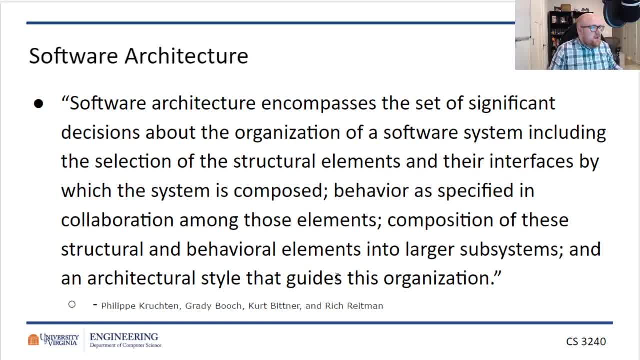 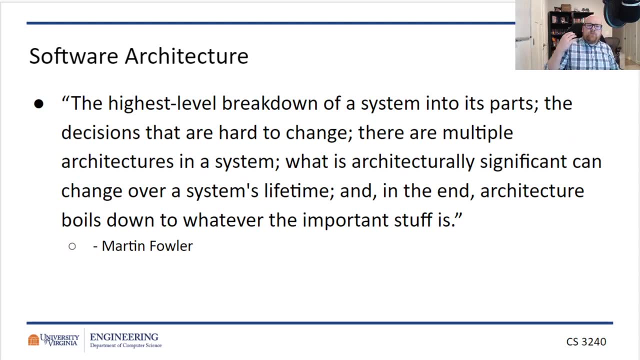 That is, how do these systems interact with each other? and is the composition, that is, the building of the structural and behavioral elements into larger subsystems and an architecture that guides this organization. Now that that quote seems really hot and heavy there. More broadly, It's the highest level breakdown of a system into its parts. 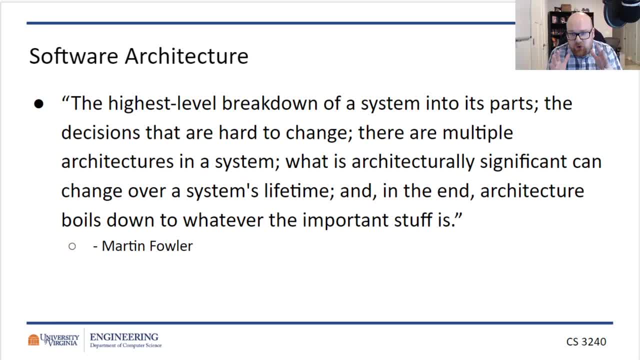 The decisions that are very hard to change, because we because we're talking about how the system is going to be laid out at core, at the, at the root design level. We're talking about the broad organization of the system. It's very hard to change this later. 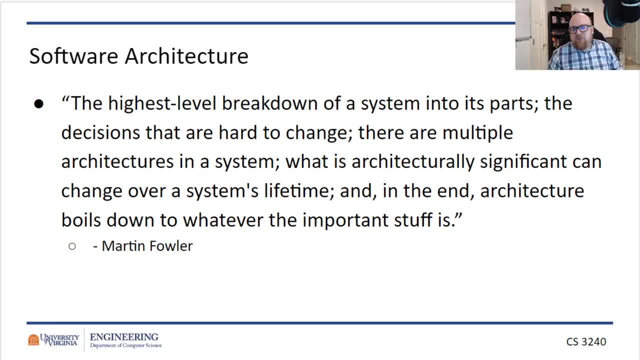 You can't say, oh, we're going to build a skyscraper, and then halfway through say, now forget the skyscraper, Let's, let's just build It really really wide instead of really really tall. You can't do that in construction, right? 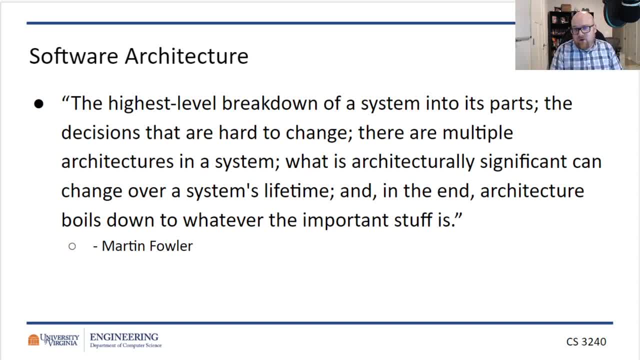 You started to build the skyscraper. You're stuck with the skyscraper. Now you have to shoehorn decisions into a skyscraper that may not actually fit particularly well there. So we're talking about architecture, We are talking about what is the overall organization of the system, and we want to get that question right. 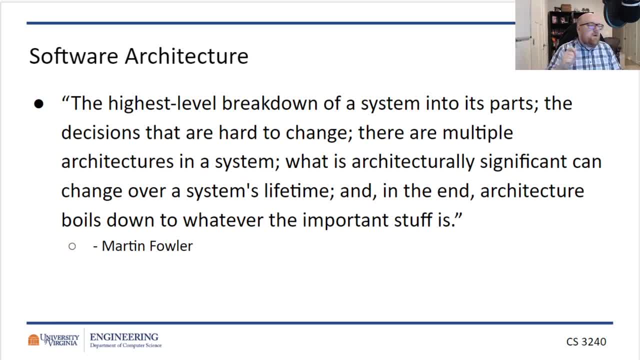 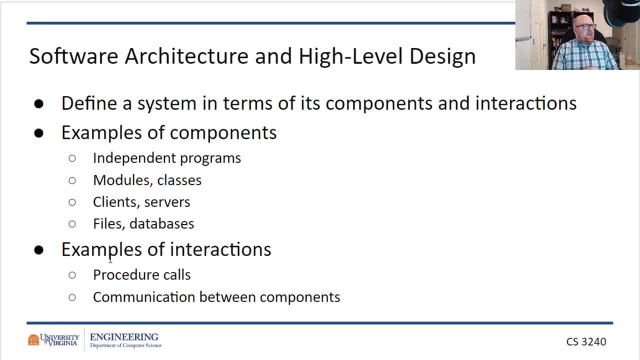 Because if we get that question wrong, it's going to be very, very hard, Hard to change it later. This is the first design decision and it's the most impactful, And so, when talking about high-level design, we define a system in terms of its components and interactions. 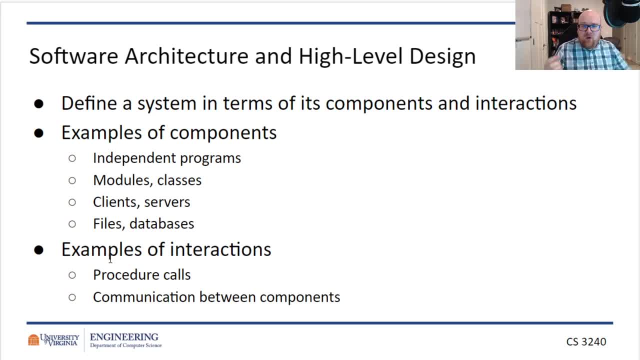 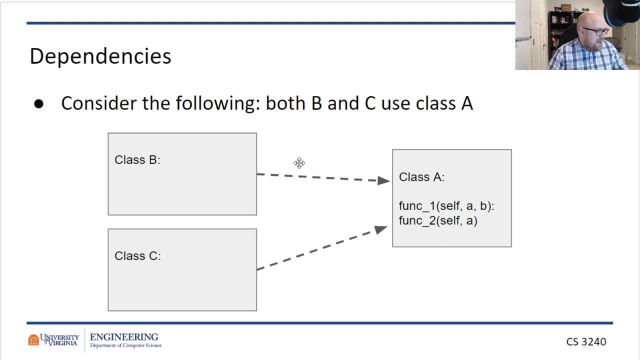 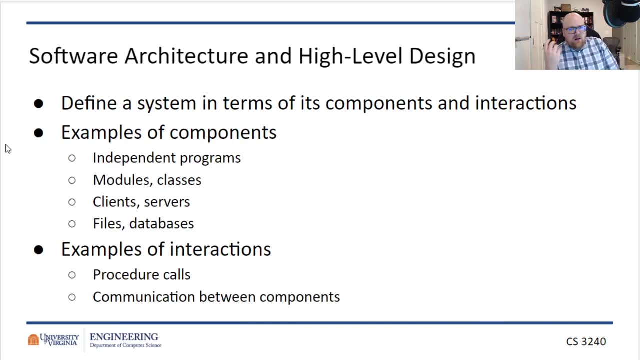 So maybe that's your classes and their API and how different classes depend on each other. I gave kind of an example of that here with this hypothetical classes interacting example And we can think of components within the system as either individual classes or collections of classes. 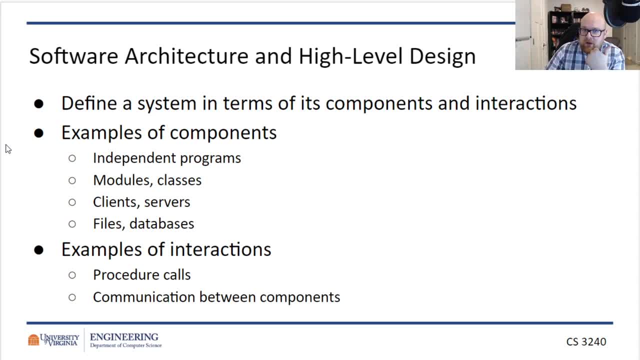 So, for instance, you can have an independent program as a component, Like maybe your, you know, using login through Google, through Google login, in order to set that up. That's an independent program. You can't change that, but you have to incorporate that into your system: different groups of modules and class. 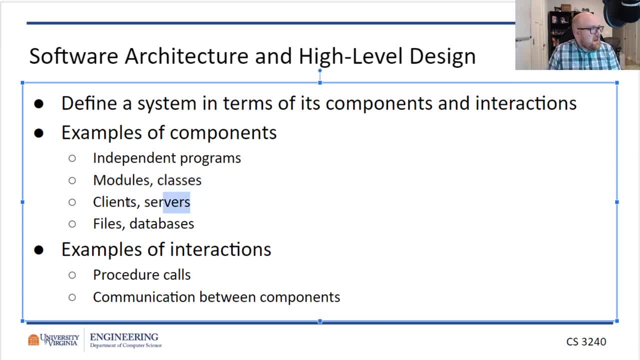 The perform a task can be an example of a component. A client or a server can be an example of component. Files, databases, examples of components. And the idea of the architecture is how do we make these things interact? Interactions can be calling procedure from a class or from an independent program. 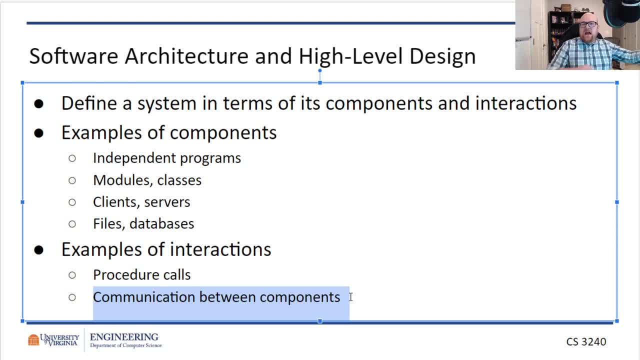 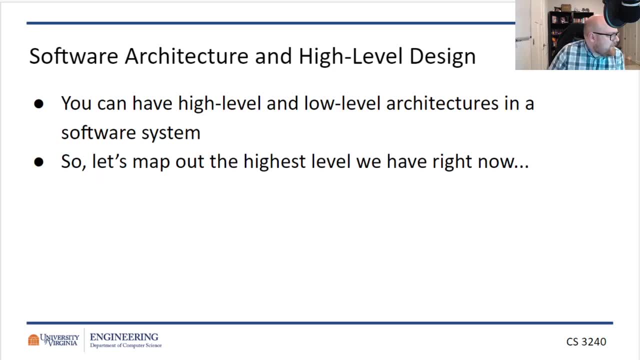 or it could be communication between the components: One class communicates with the database, or one class communicates with another class, etcetera. that's what we mean by architecture, and you can have a high level and a low level architecture in a system. you can say the overall thing is structured as a mvc, but individual components 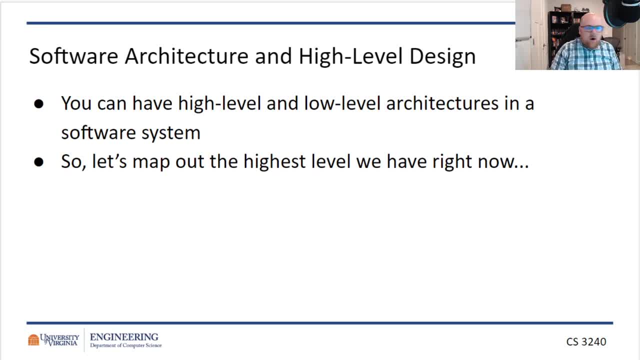 are three-tier architecture, whatever, but let's think about it right now. i want you to take a second and think about how you would describe the architecture of your system. so far, pause the video now. some of you may have found that question hard to answer because, after all, you're used to. 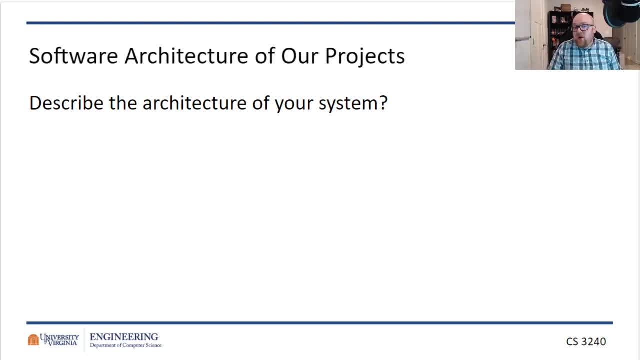 you know, building quick, disposable projects for the purposes of classes, right, the quick disposable software. and so you haven't really had to think about architecture. in fact, in 2110, we, we told you what the architecture was. i know, in in 1110, you didn't even have to worry about architecture at 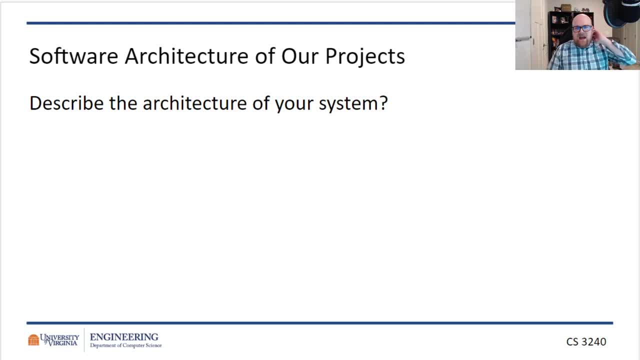 all you, you only had a single program, you didn't have multiple classes and you didn't have a interacting. so what is the architecture of a system may be a hard question for you to answer, because you you haven't ever thought of it necessarily before now. the first question is: 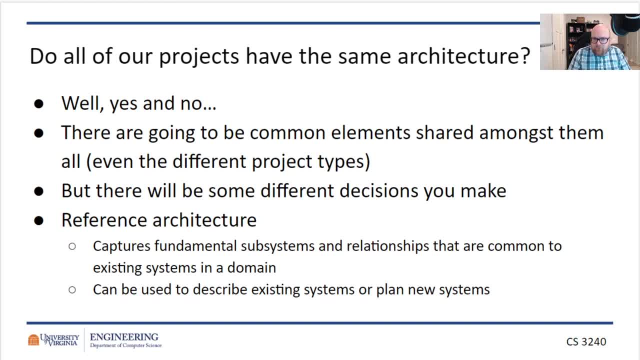 do. all your projects need to have the same architecture, and i'm shrinking my face there a bit. uh, you know i'm crushing your head. i'm crushing your head. no, um, there are going to be common elements among projects of even different types, but you will be making 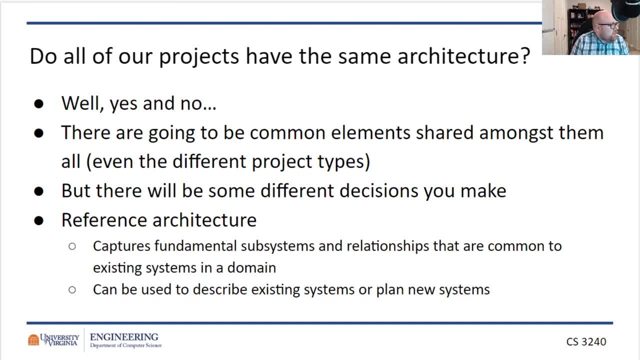 different decisions. so we're going to talk a bit about reference architecture here in a second um, the reference architecture of how web apps are often made, and this captures the fundamental uh relationships and subsystems that are going to be existing pretty much in any system: in, in, in. 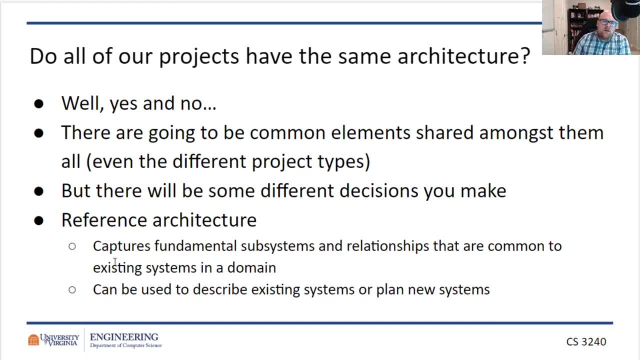 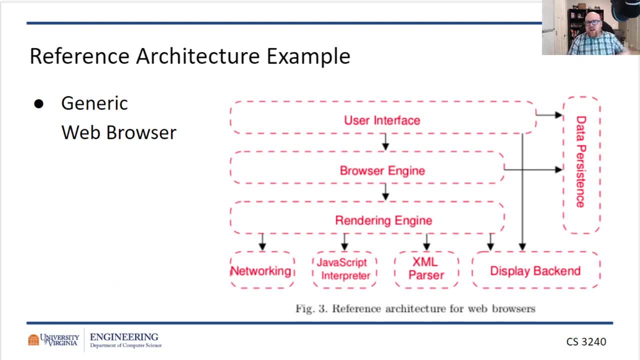 any domain that you're building with with, say, a web app. um, so this is the reference architecture of how web apps are often made, and this captures the fundamental reference architecture. example: uh, and this is a generic web browser and different web browsers implement this differently, but the idea is the user interface. that's what you're seeing on the 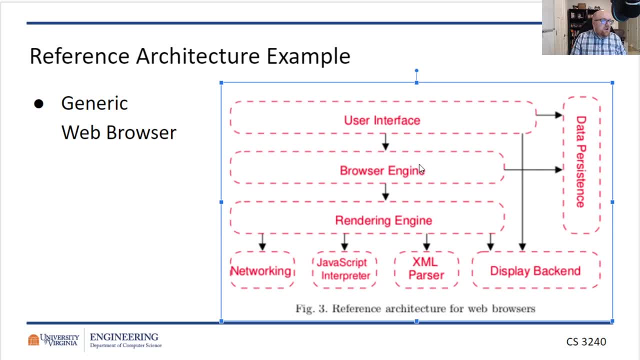 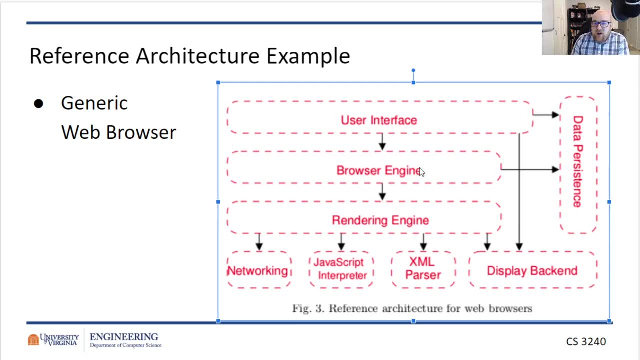 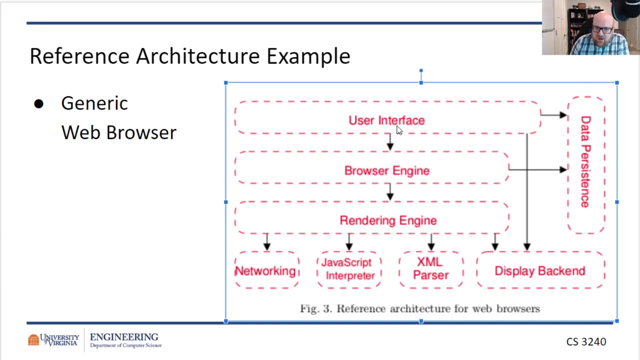 screen. that's the top level that uses the browser engine. but the nice thing is, if the user interface changes, we don't actually have to change the browser engine. that's actually a pretty advantageous thing. going back to our example about dependencies, the user interface depends on the browser engine, not the other way around, and since the user interface is likely to change to meet, 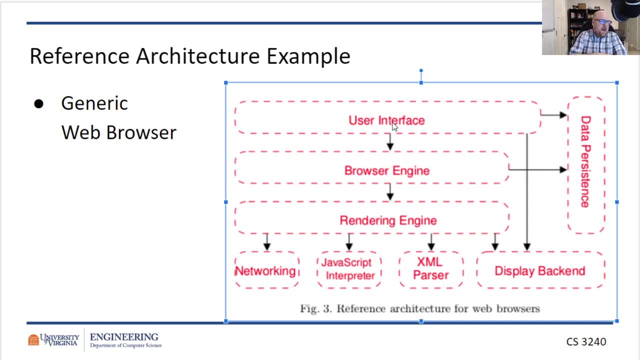 particular needs. it's helpful to think of it as a separate entity. we have, broadly, a user interface that works with the browser engine. the browser engine works, uh, it works with the rendering engine that actually produces the display. it uses, you know, all these different tools to produce what. 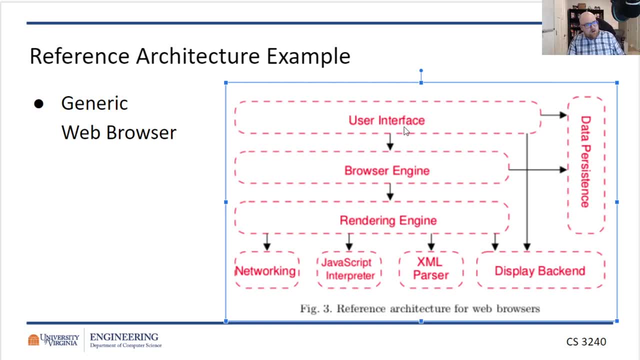 the user should see drops into display backend, which the user interface references to pull up. then from there the user and the browser may both work with some particular shared set of data, and this is a generic web browser architecture. broadly, you can see here that we have mozilla and if you're not getting what every single one 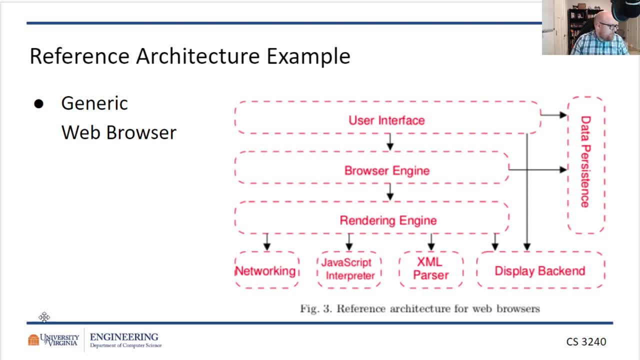 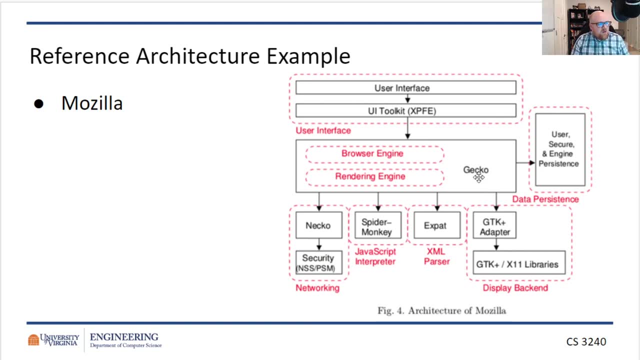 of these things does. yet don't worry too, too much yet. uh. so here, for example, is mozilla, here's the user interface. inside of gecko is both the browser engine and the rendering engine. we have systems that deal with communicating over the network, systems that do javascript interpretation, systems that parse. 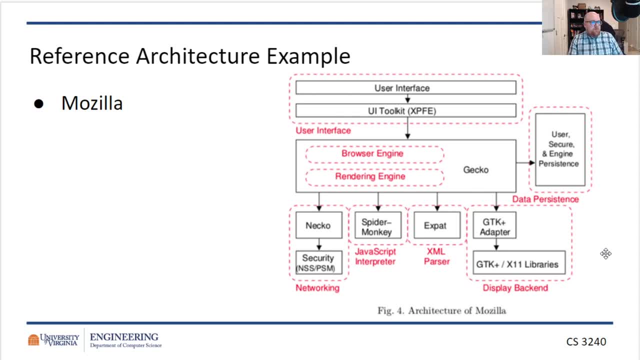 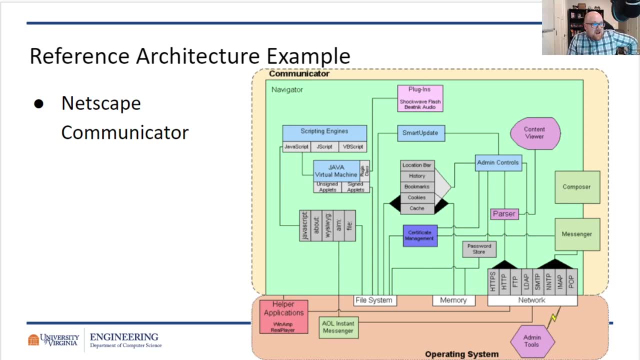 xml files or data, or data files, um, etc. netscape- this one's a lot more complicated, netscape navigator, and it's a lot older, and it's why, uh, we don't use this much anymore. not a lot of systems are built with that in mind, but most likely, you probably weren't thinking of an architecture like this. 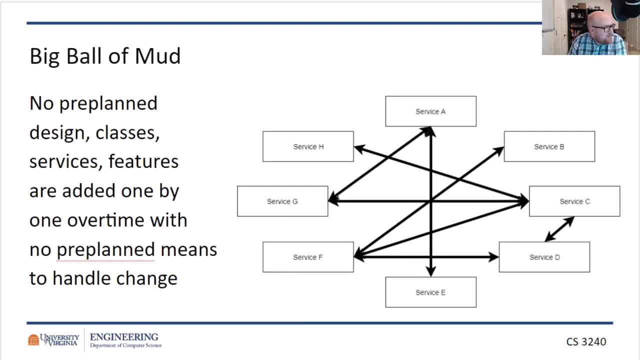 most likely, your architecture probably looks something like this. so far, although you may, you probably don't even have this many services yet- and this is called a big ball of mud, and a big ball of mud is what we would call an architectural anti-pattern. we're going to talk about architectural patterns here in a second. the idea of a pattern is it is kind of 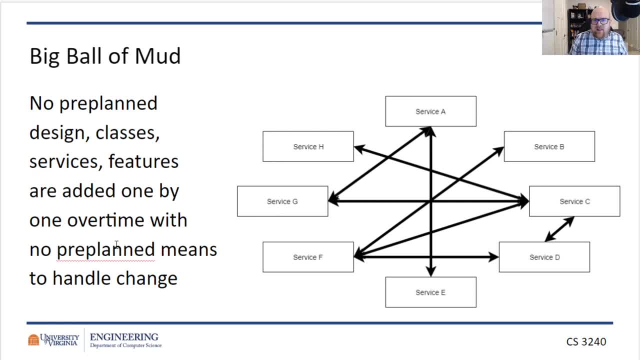 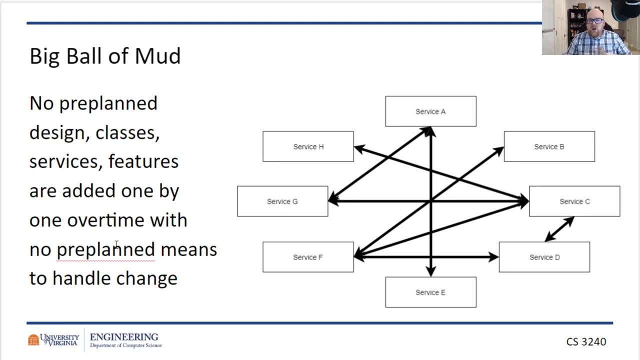 because it doesn't do any of those things. the big ball of mud is this: you add classes as you think of them, pardon me. you add classes as you think of them. you add services as you need them, and you don't really pre-plan an adventure. you add classes as you think of them and you don't really pre-plan an adventure. 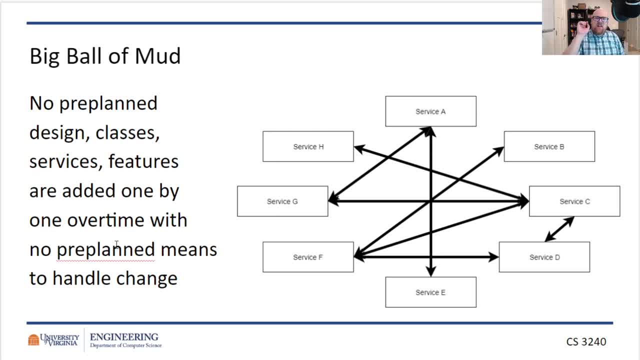 where they are going to go. you just kind of slap them on. think of it kind of like sticky notes. you just put it on the surface. the problem with the big ball of mud is that it has basically no thought in the future to how the system will evolve over time and as a result of that you end up with a lot. 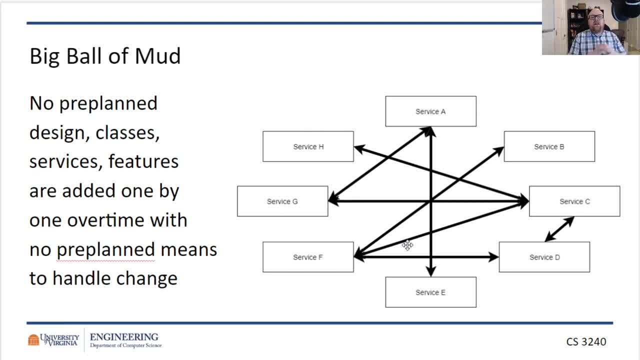 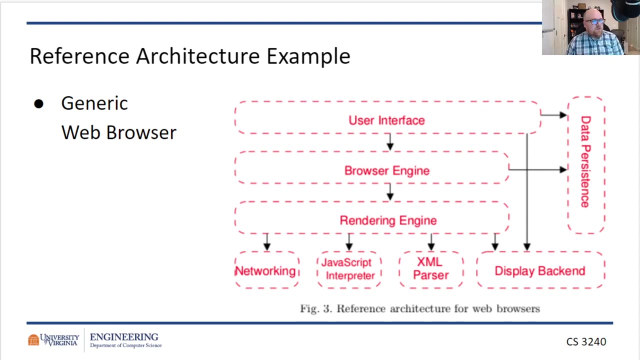 of interdependencies, you end up with a lot of classes depending on a lot of other classes and one change will necessarily propagate very far and wide and it can make the system even even more expensive to maintain later on. this leads to higher entropy, whereas something like this reference architecture- this would be say a reference architecture to a generic web- 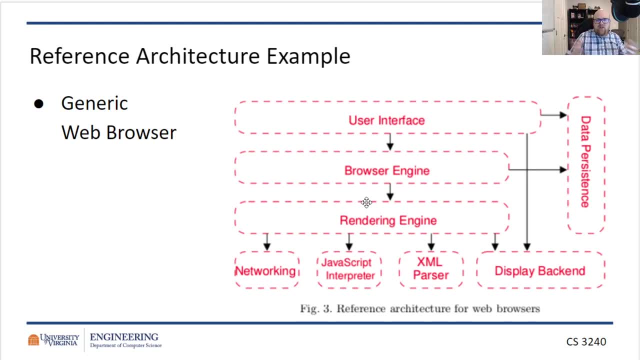 browser by planning out how the system is going to react. broadly and again, these components are may not be individual classes, they may be groups of classes, services. whatever the point is, by planning to organize these things in this way and by making sure that we have one directional dependencies, we can limit the. 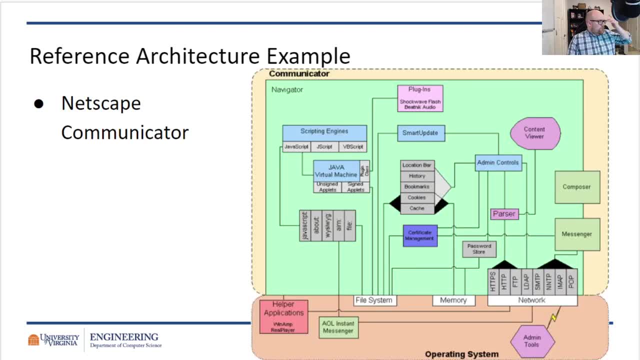 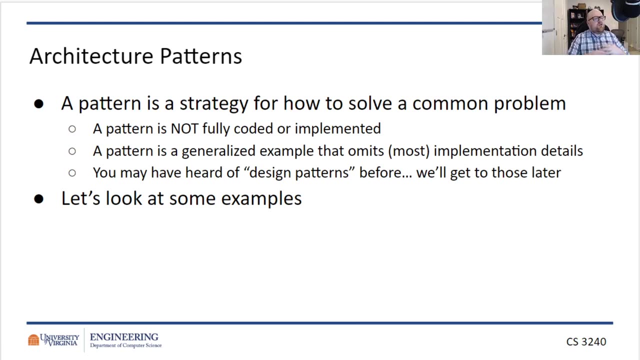 propagation of changes, um, you know. so that's why, when we talk about netscape navigator, like yeah, this is bad, it's full of tons of interdependencies, it's hard to read and it's really hard to understand what you're doing, for that very reason. so an architectural pattern. 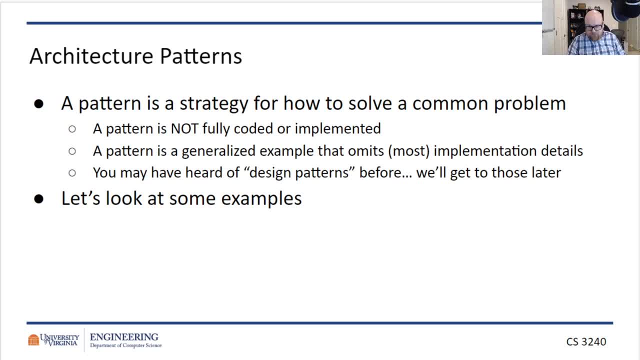 is a strategy for how to solve a common problem. i have these components that i want to combine. it is not a fully coded or implemented system, rather it is an idea. it is a pattern that omits the implementation details. it's intentionally vague, but that's because you think of the pattern. 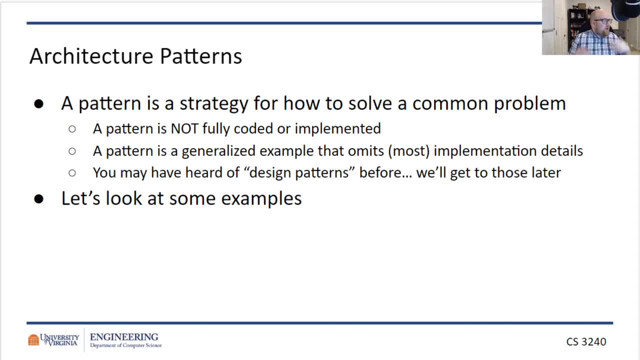 as the idea that you implement um. so that's why i'm saying it's a pattern, that's not a full coded. there are some examples of patterns in architecture. there's also design patterns- how we organize specific components or specific features- and we're going to definitely talk a lot about design. 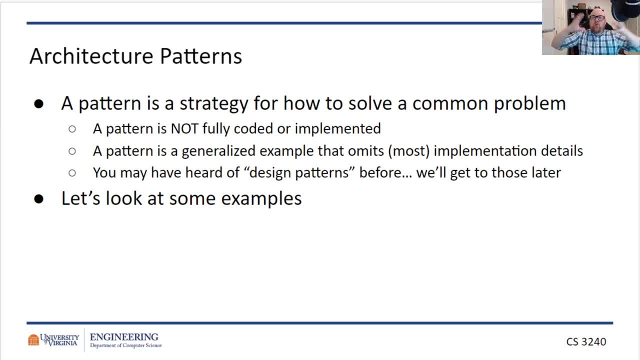 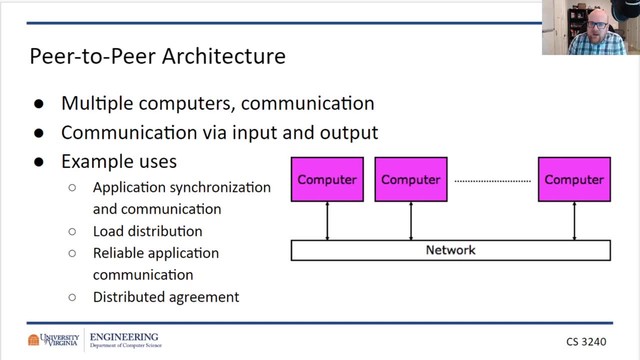 patterns, but architectural patterns are just broad organizational structures for the system. an example would be something like a peer-to-peer architecture. the idea of a peer-to-peer architecture is you have multiple computers communicating with each other over some shared network. often that shared network is the internet as a whole, the world wide web, and so you communicate two. 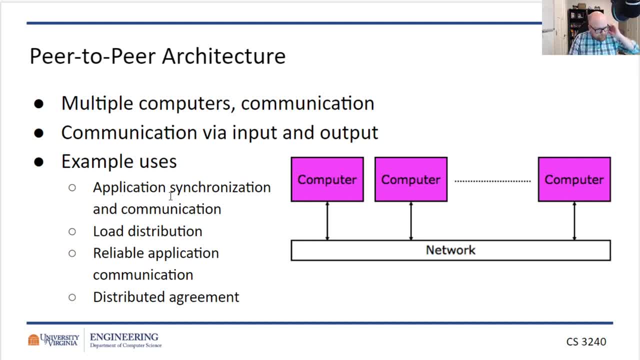 other systems via input and output and this allows um. you know, you can synchronize different applications. you can distribute the load of the system. so if you have a system where you need a lot of individual systems interacting together and you want to distribute the load of some work and you want to have some agreement with 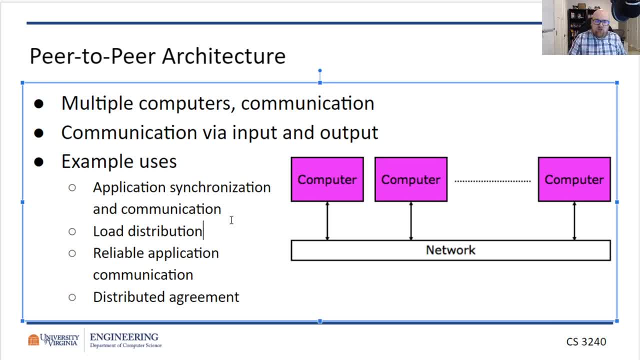 how that's distributed. you may use a peer-to-peer architecture, where you have some network that computers are communicating with each other over, and you will design the app by designing what features are the computer doing? what is the input and output to the network that the computers are going to perform? a layered architecture is the system is provided. 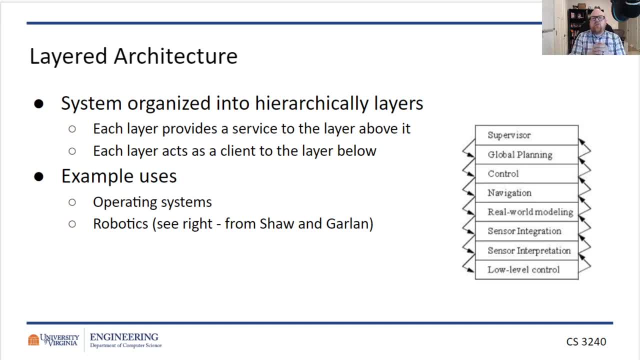 with a core system and it's created to Verkehr architecture. so if you have a Kalau architecture or is organized into hierarchical layers, each layer provides a service to the layer above it and each layer acts as a client to the layer below. by what i mean service and client? if you go into 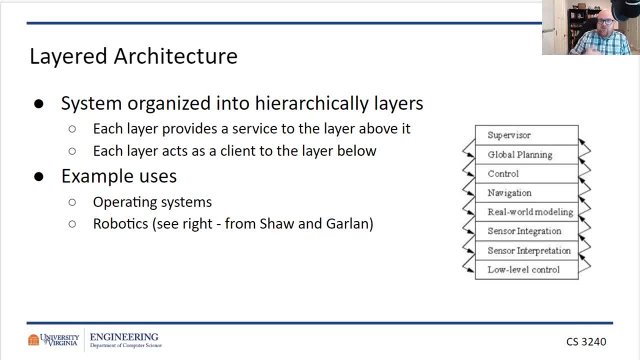 a restaurant and order food, you are a client. if you are working in the restaurant bringing food or cooking food for the client, you are the server. so the idea is there's some supervisor that uses our pardon me. a supervisor is a client to global planning and global planning is a is a service for the. 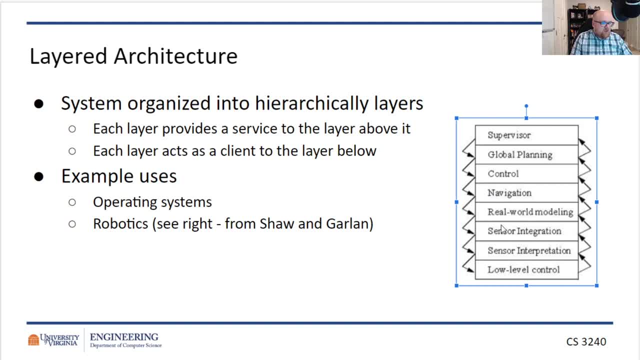 supervisor, control, navigation, etc. so low level control is a service used by sensor interpretation. so this might be for, say, a robotic system. the supervisor in this case, by the way, is not a human, it's just the over over working, uh, high level program that that's managing everything below it, albeit indirectly. 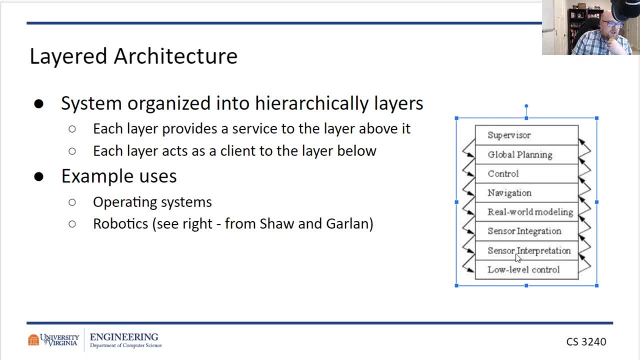 so the low level control. this is uh used by the sensor interpretation and it feeds information back to sensor interpretation. but the key is, the supervisor is not aware of control, the supervisor is not aware of navigation, the supervisor is not aware of real world modeling, and so on same way, real world modeling is very 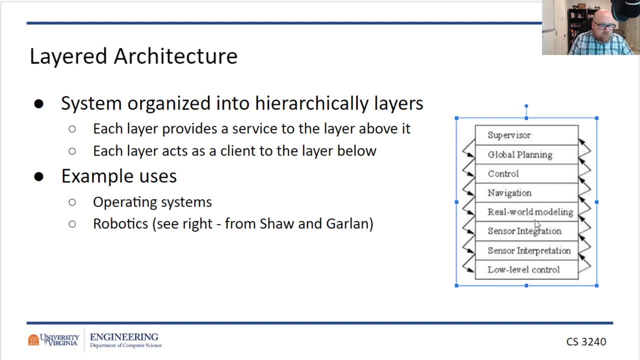 important to the supervisor. so the supervisor is not aware of navigation. the supervisor is not aware of the navigation module and the sensor integration module, but it is unaware of the modules outside of its scope. this makes each system easier to design and build because if change- if i need to change- the interface of real world modeling, then certainly that's going to. 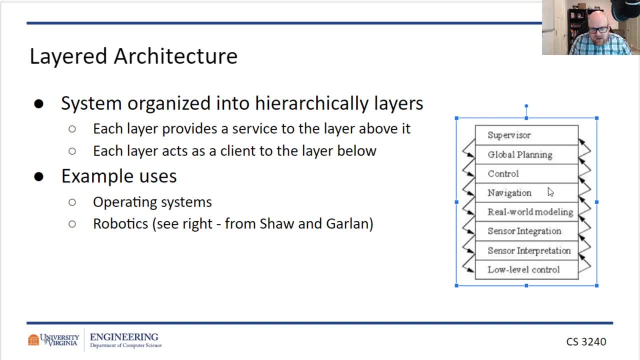 affect navigation because navigation is going to have to update to that changed interface. but if navigation can update without changing its own interface, its own set of features, then control would not need to change. because we made a change to real world modeling, we can stop the propagation. think of it, you know again, like those ripples in 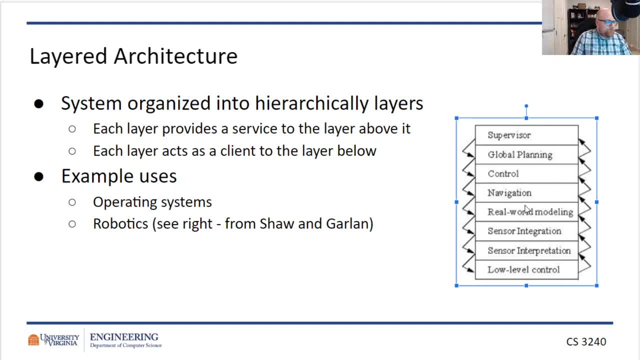 the pond, but we stop them somehow, we prevent them from propagating further, and this idea is at the basis of um, this layered architecture. there's n tier or n layered architecture where n is the number of layers, and a common example of that is a three-tier architecture where at the top, 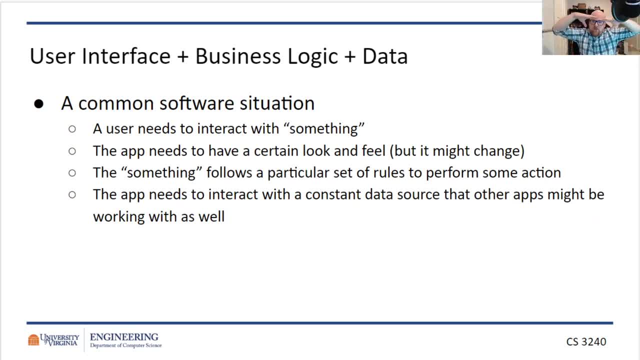 we have the user interface and the user interface is a client for the business logic and the business logic is a client for the data. data provides information to the business logic. the business logic provides some subset of that information or some modification of that information to the user interface. so the user 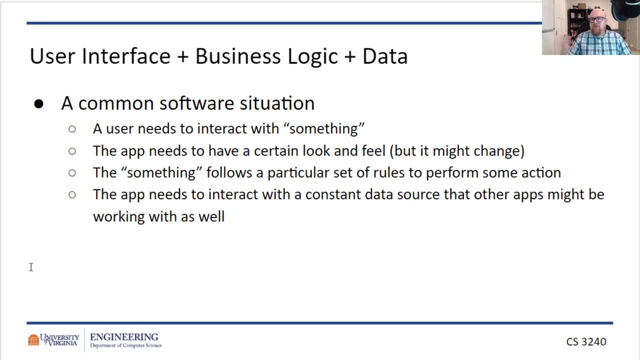 interacts with something- a web browser, a form, command line, whatever. this allows us to design an app that has a certain look and feel but could change. they just change the layout of facebook. i hate it, but they can do that because they do some type of design like this: the user interacts with that something and that something follows a. 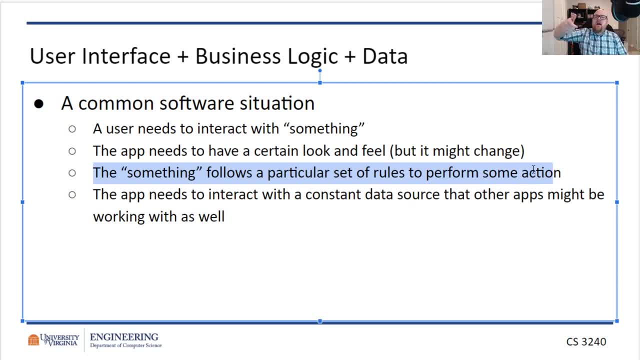 particular set of rules to perform an action, and that's what we're going to do today. that is to say that it interacts with the business logic layer and the business logic layer follows those rules or standard operating procedures, or whatever you want to call them, follow some process to gather information. where does that get the information from the business? 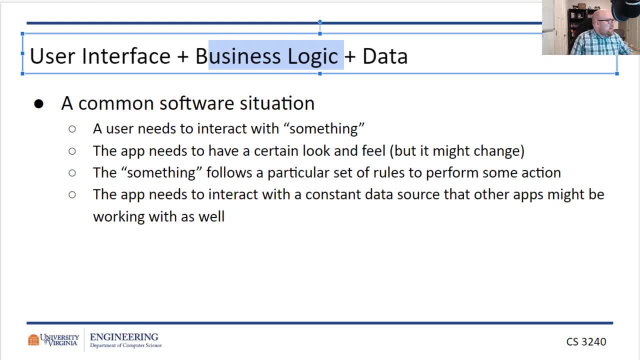 logic layer interacts with the data layer, so if i were to illustrate this i might do something. and we're we're working live with shapes in google present so broadly, and again this gets into a layered architecture. we have the user interface layer, sometimes called the presentation layer. 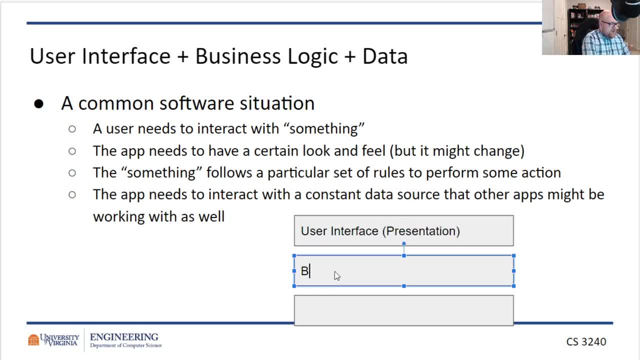 we have the business logic layer and then we have the data layer and sometimes, by the way you'll you'll see this also called the controller layer or just or just logically layer. you'll see it called different things, but the idea is the same and the idea is the interface. 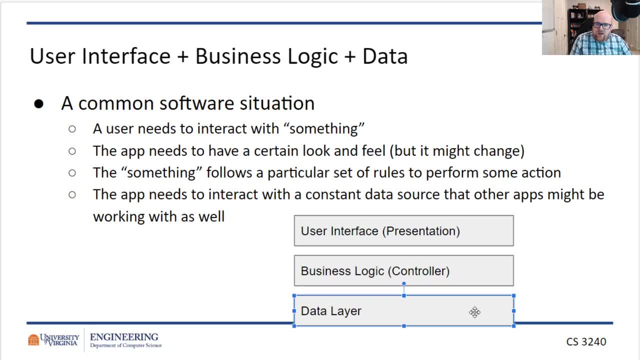 uses the business logic layer and the business logic layer uses the data layer, but the user interface does not directly use the data layer. it never directly interacts with data, and the advantage of this is that the data layer may be something that changes. maybe, instead of using files, you switch to a live database. well, now you definitely have to make 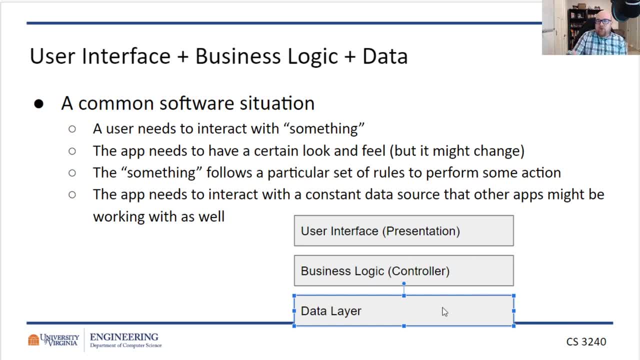 changes to the data layer and you're you know you're gonna have to replace all that file io with sql queries, right, but if you can preserve the same interface, that is, you change everything like it's like. imagine you have a house, right, and someone remodels the entire inside of the house. 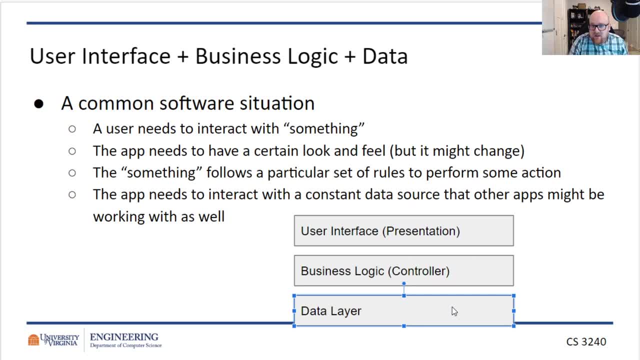 but they keep the outside looking exactly the same. you know, then? that's what i'm talking about. if data layer can change its implementation details, go from file io to, say, a live database, without changing its interface, then the business logic layer is completely unaware of the change. 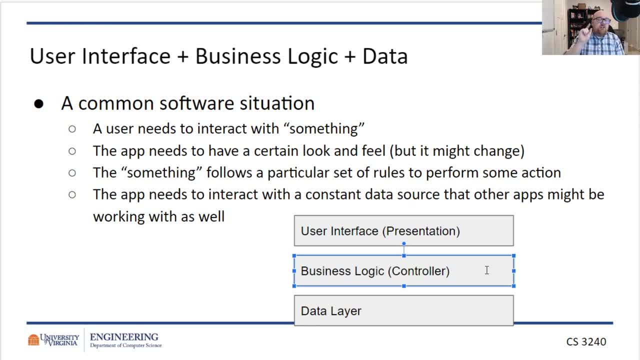 and the change never even propagates there. if the change does necessitate a change to the interface, data layers interface has to change. maybe we need a username and password and address for the database? okay, so the business logic layer will need to be updated. but again, if the business 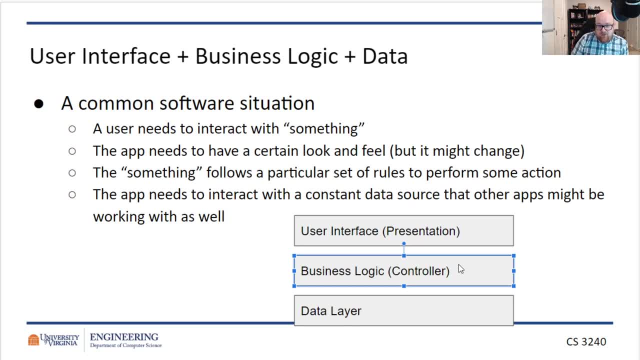 logic layer can be updated without changing its interface, then we don't need to ever update the user interface in this case. So everything uses the thing below it. but the advantage is in a layered architecture the data layer doesn't even need to necessarily be aware the controller layer. 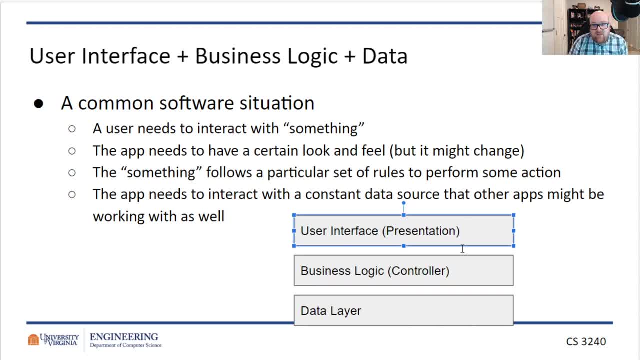 exists. A change to the user interface will not necessarily result, and almost never will result, in necessarily changing anything in the next layer, down Changes tend to. you can have a change that propagates up, but it's much less likely to propagate down. Why are we spending? 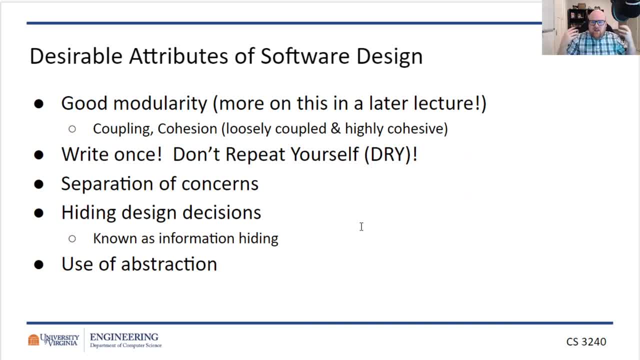 all this time talking about this Because we want to have desirable attributes in our system, because, remember, we want to make our software modifiable. We want to have as few ripples in our pond as possible every time. So, in order to do this, we need to have good modularity, which we will talk about. We'll talk. 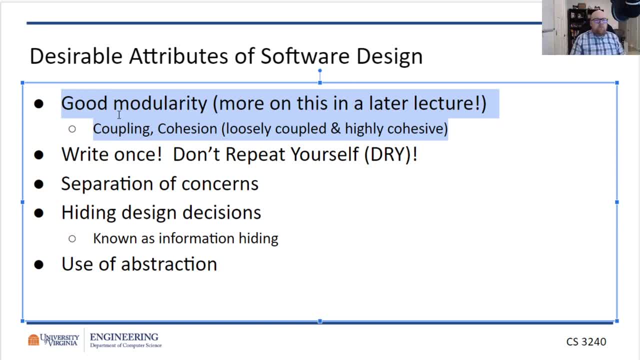 about it. I promise you. We want to be dry, so you want to be dry as opposed to wet. Write everything twice, write everything thrice, etc. You want to write something one time. We want to separate our concerns. The idea is each component should deal with one concern or one subset of concerns. It 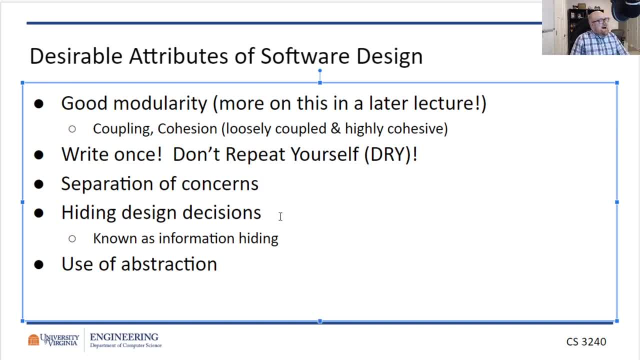 shouldn't deal with one set of concerns. It shouldn't deal with one set of concerns. It shouldn't deal with everything. You want to hide design decisions. By that I mean you may be thinking: wait, we just spent a lot of time modeling design decisions. We're not talking about hiding it from. 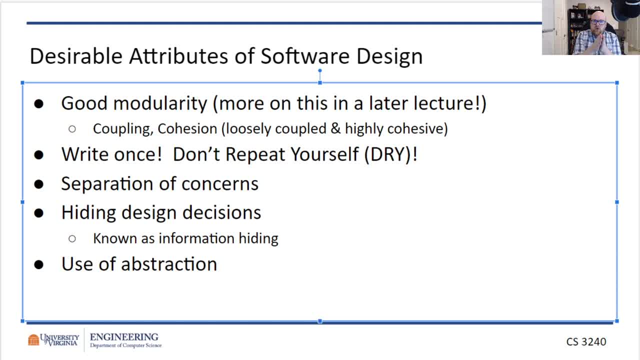 the developers. We're saying that one class should be as aware of the rest of the system as little as possible. In order to design our system well, we want as few dependencies as we can have. We will necessarily have to have as few dependencies as we can have. We will necessarily. 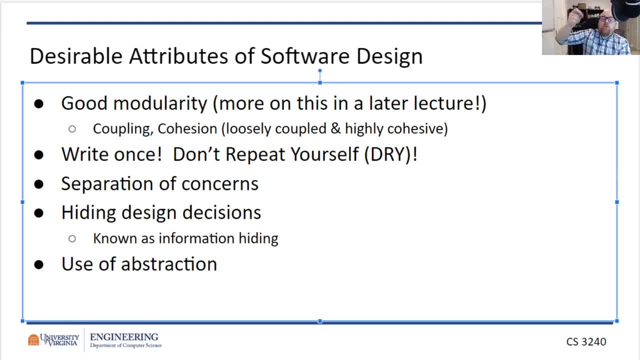 have as few dependencies as we can have. We will necessarily have as few dependencies as we can have. We will necessarily have dependencies. The user interface will necessarily have at least some dependency on the data, If not direct, then at least indirect. We're going to have dependencies. 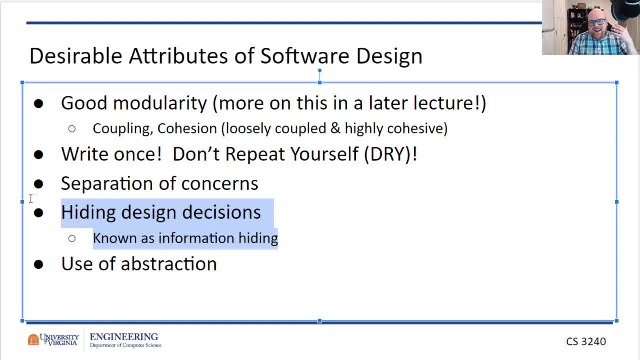 Can we limit those? By limiting them, can we make it such that one system being changed propagates as little as possible? We're going to look at these examples later in a design lecture, but I just want you to know that the idea of peer-to-peer architecture of layered 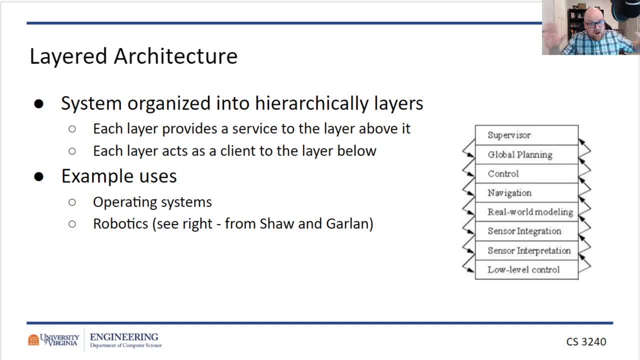 architecture of MVC, which I'm not talking about in this lecture: model-view-controller- that's going to be next week. That model-view-controller is another architectural pattern. That is a pattern that was formed because it's useful for achieving these things. 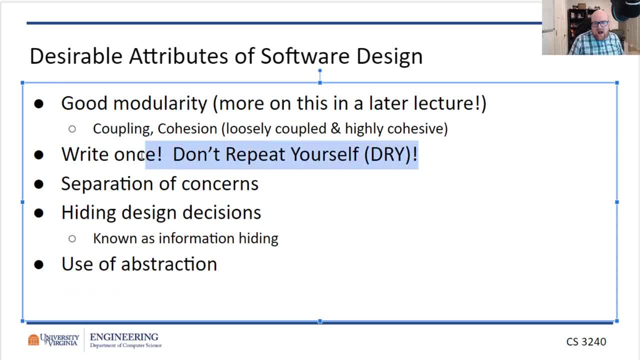 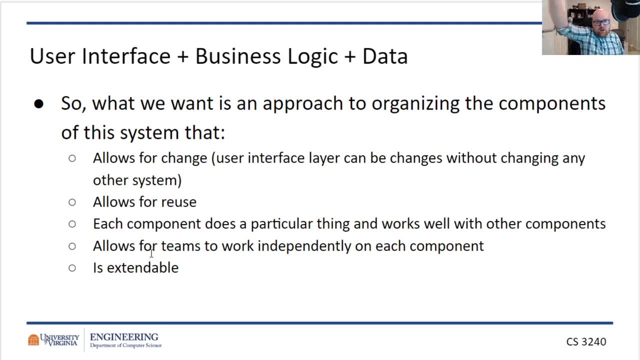 Good modularity, ensuring things can be dry as opposed to wet, separation of concerns, etc. So, going back to our three-tiered architecture: user interface, business logic and data. this allows for the user interface to be changed without changing any other system. 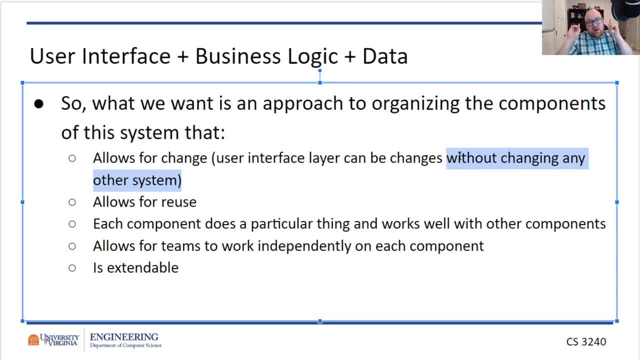 That's huge, because the user interface may change a lot. It allows for reuse of components. If I want to access a database, I only need to get a student with a given id number. tudo lo کے знographers mit einem gewissen idaster soils. 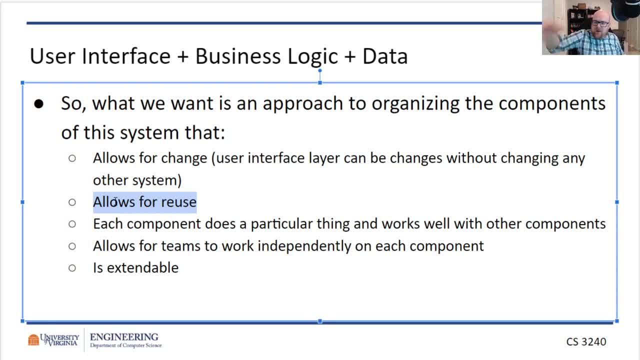 I only need to write that feature once in the data layer And the controller layer. if it has multiple features that need or the business logic layer —excuse me that- multiple features that need to perform that action, It can call that same action, not re-implement it. It allows teams to work independently, regardless of how big the enterprise. For instance, about a mom and a dad and it's all, Amanda, but imagine you have a baby on your shelf and everyone's in your quarters. based on the Hammero дух. 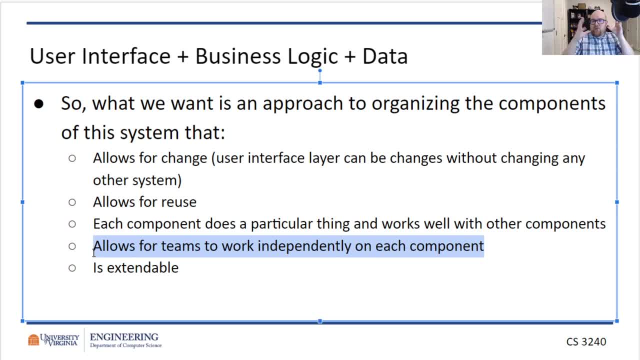 work independent on each component. The user interface team can be separate from the business logic team, can be separate from the data team and it's extendable, That is to say, it's easily changeable. We can add more layers if we need to. Why three layers? Why not four? if we feel that we. 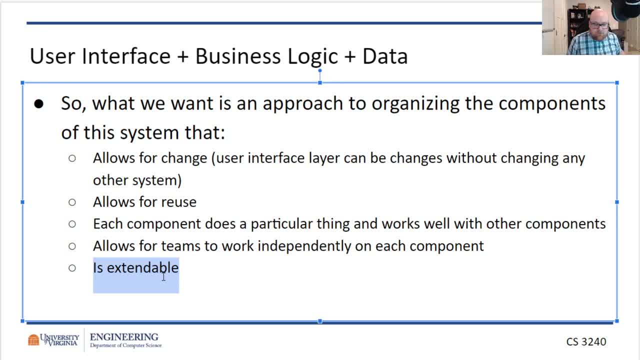 have valid design reasons to do so, But it's also just easily modifiable over time. So we will talk a lot about MVC, which I didn't mention, is another architectural pattern. We're going to talk about that a lot next week, But the next video I'm going to put out and I will put this: 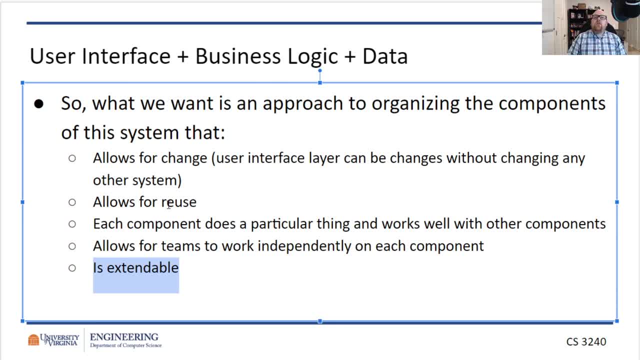 out very, very shortly is going to be looking at an example of three-tier architecture in Java and actual implementation of it. It's going to be a very rough, simple implementation, but it's just designed to show you the advantages, to show you what we mean. 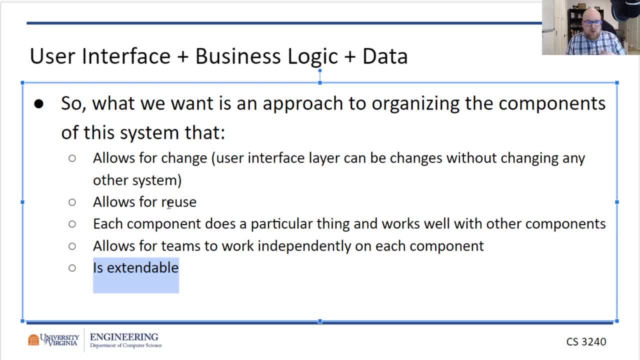 very practically at a code level when we talk about things like reuse, when we talk about allowing for change, etc. So I hope you watch that video when it comes out. I hope you enjoyed this one and thank you for watching. Take care.